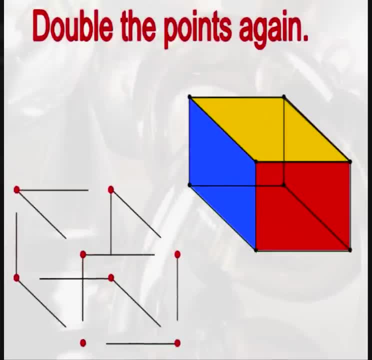 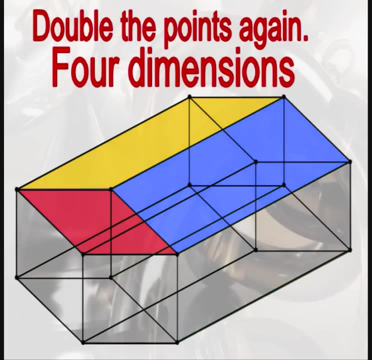 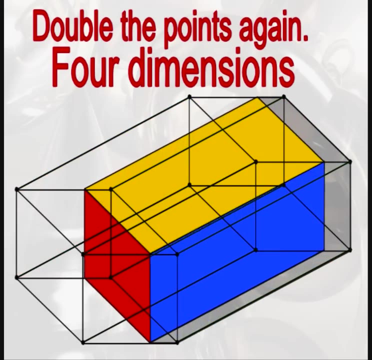 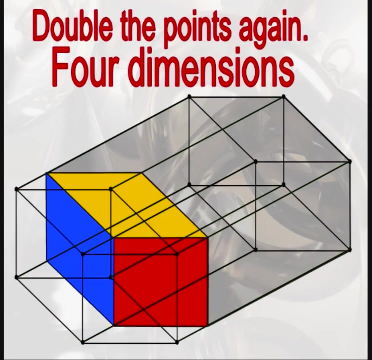 Double the points yet again, and you have four dimensions. Double the points yet again and you have four dimensions. Double the points yet again and you have four dimensions. Skeptical, You're watching this on a flat two-dimensional computer monitor. 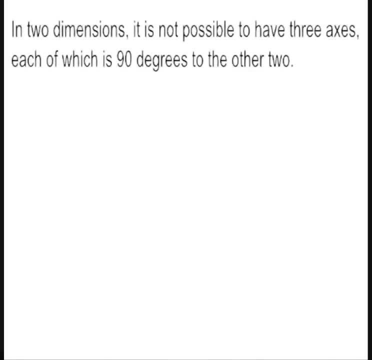 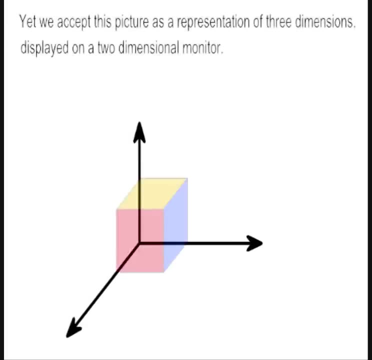 In two dimensions, it's not possible to have three axes, each of which is 90 degrees to the other two. Yet we accept this picture as a representation of three dimensions displayed on a two-dimensional monitor. In three dimensions, it is not possible to have four axes, each of which is 90 degrees to the other three. 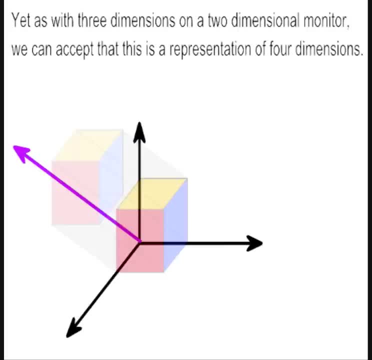 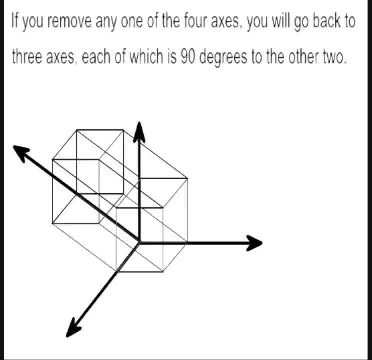 Yet, as with three dimensions on a two-dimensional monitor, we can accept that this is a representation of four dimensions. If you remove any one of the four axes, you will go back to three axes. If you remove any three axes on a two-dimensional monitor, you will go back to three axes. 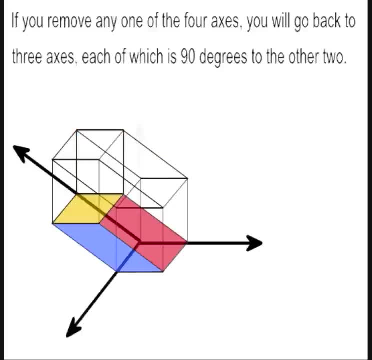 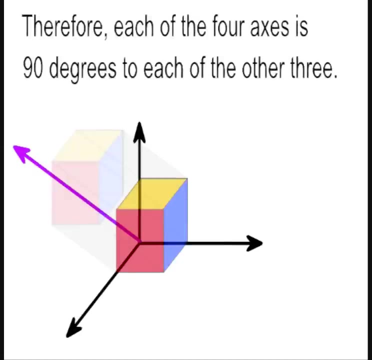 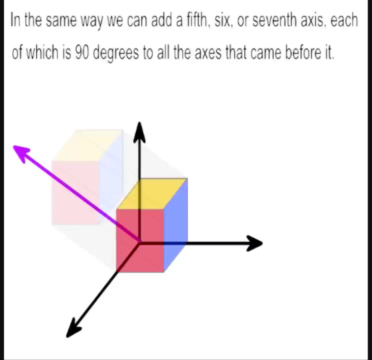 Now check out willgif. We push the button when we see a version of the two-dimensional model. Therefore, each of the four axes is 90 degrees to each of the other three. In the same way, we can add a fifth, sixth or seventh axis, each of which is 90 degrees.